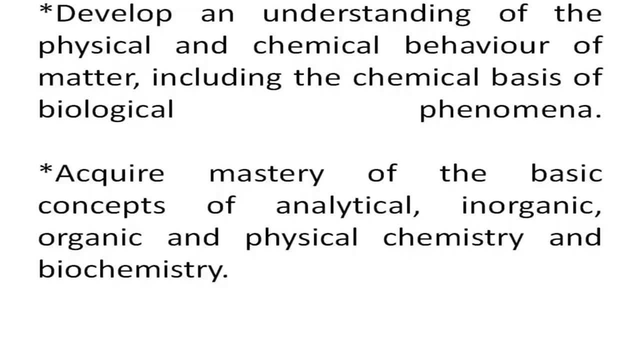 learn about the higher techniques, higher learning substances, higher instruments like LMS, MS, AAS, all this type of instrument. we want our students familiar with that. all types of techniques. Actually, in our course we have taught about the all types of new. 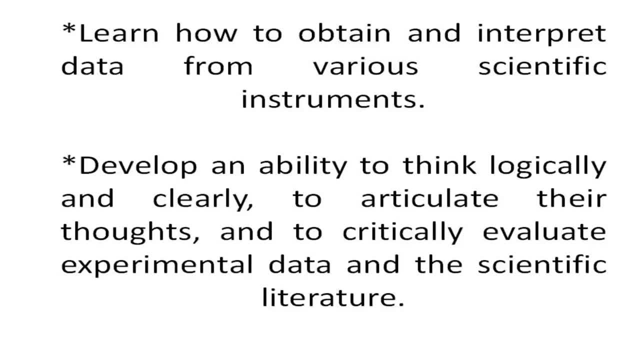 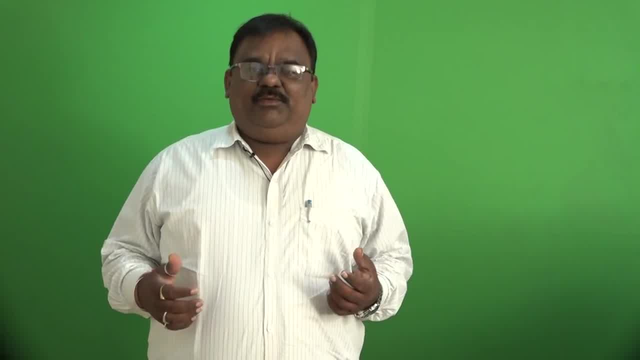 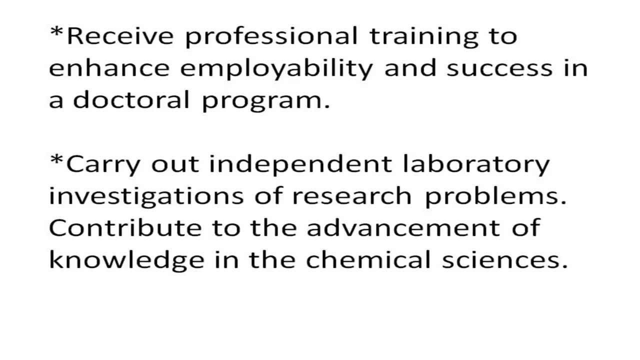 modern environmental chemistry. contents In our chemistry not only basic fundamentals of the pollutions. it is not only our Indian problem, this is the problem of global, this is the world, How we can solve this type of problem. So it is necessary to student know about the 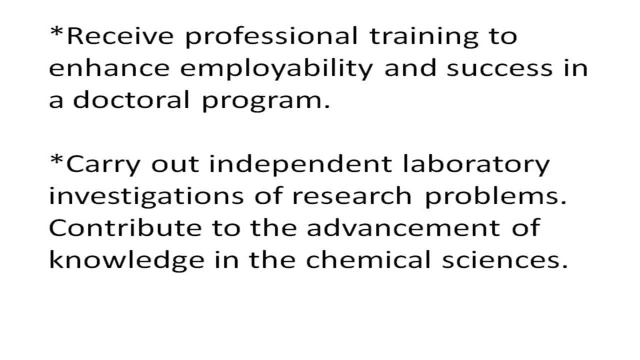 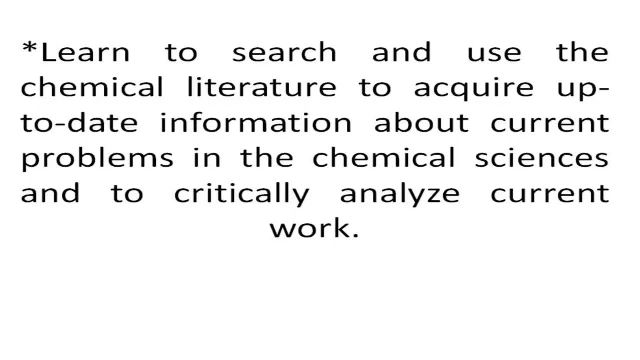 soil chemistry, water chemistry, about the atmospheric chemistry. We also teach about the toxicology: what is the food and hazardous? what is the effect of this to the student? how student learn about the all types of techniques and do the research on this type of advanced 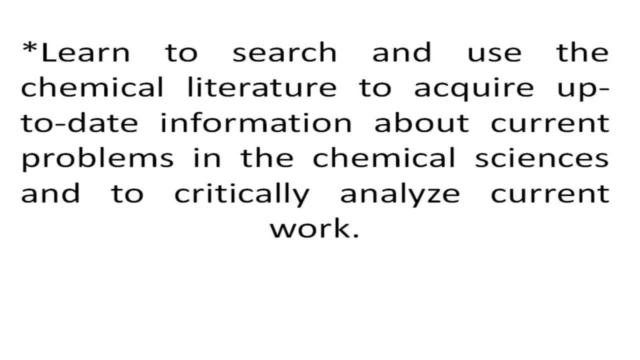 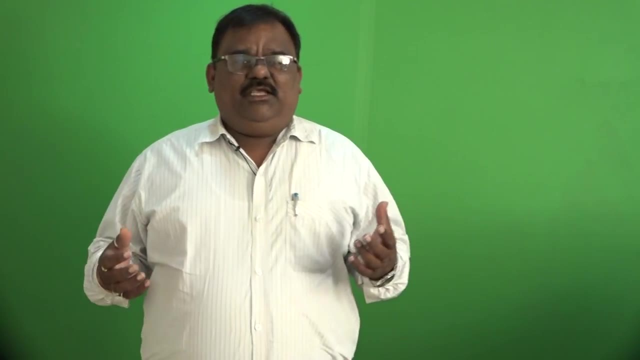 topic: Our student. Always we want to student, not only interact with the modern society, but interact with the higher research instrumentation facility. What we want, that is, the atmospheric and the hazardous effect is not only affected us, but this is the not only affect this, but 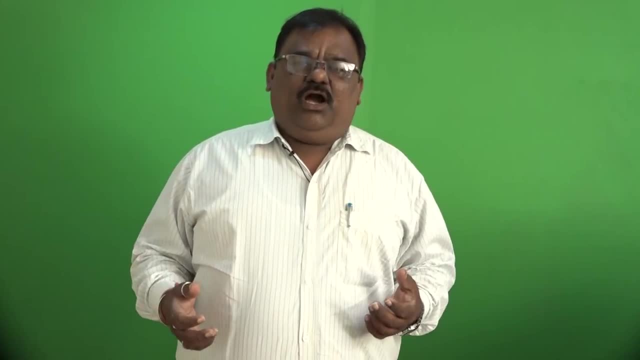 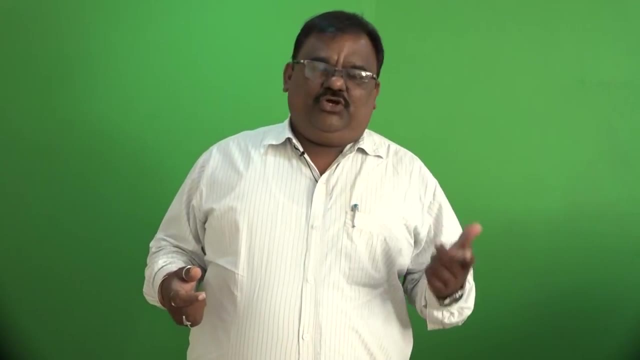 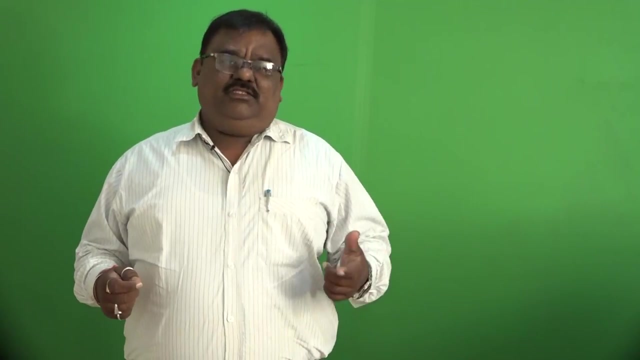 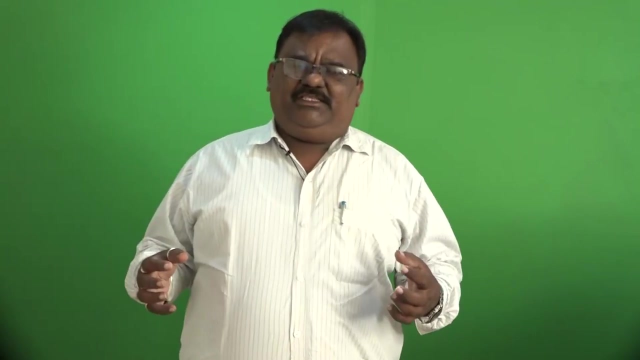 this is the loss of our world. also How we can treat this. So in our content, we can treat about the GIS system, geographical information system. We can treat about the water management, how we can conserve the water, how we can biodiversity- Biodiversity is now day by day. 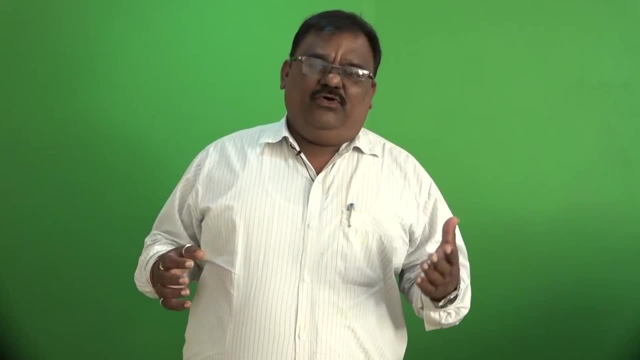 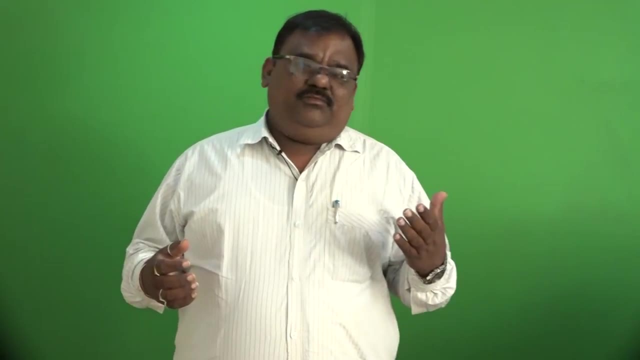 It is now just damaging to our world. How we can explain this? how biodiversity conserve this type of How water management is do by the. How we can, How we can conserve this type of How we can conserve this type of How water management is do by the. 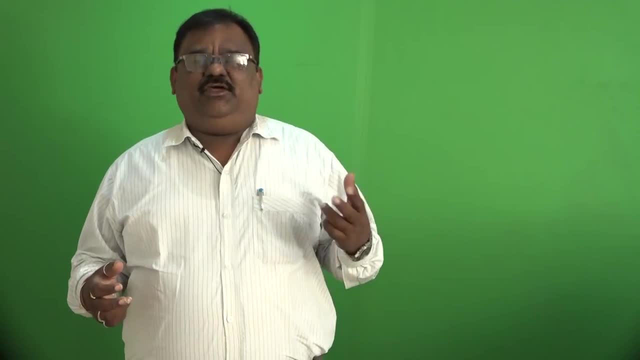 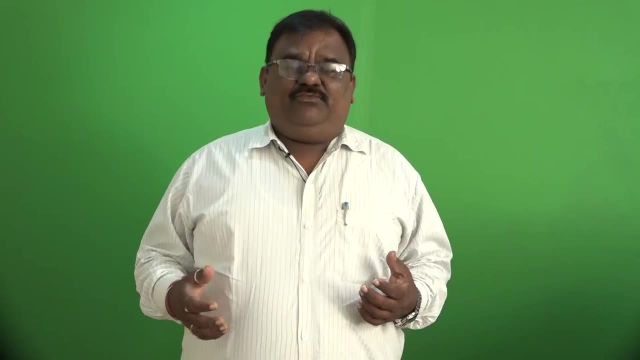 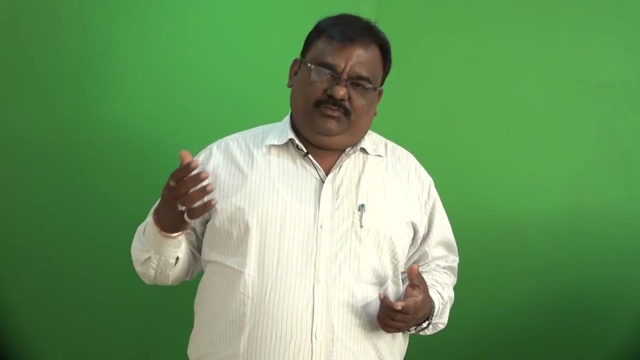 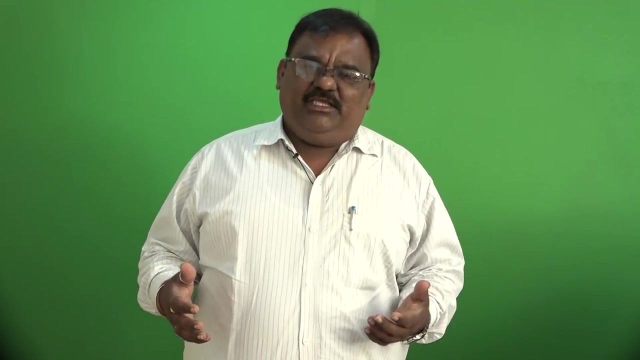 do by the student. all this is content learn. this is in environmental chemistry. in our content we also want to student learn about the green chemistry. what is the green chemistry? green chemistry is the sustainable development of the chemistry- how we can develop the without any damage to the world. what is the biotechnology biochemistry? in biochemistry we learned about the. 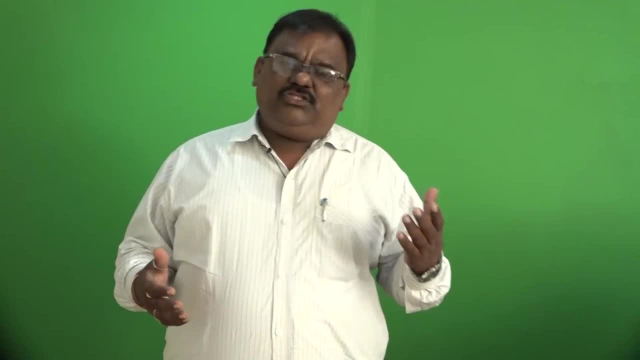 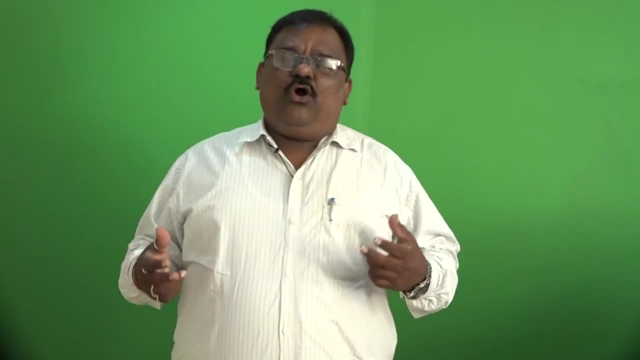 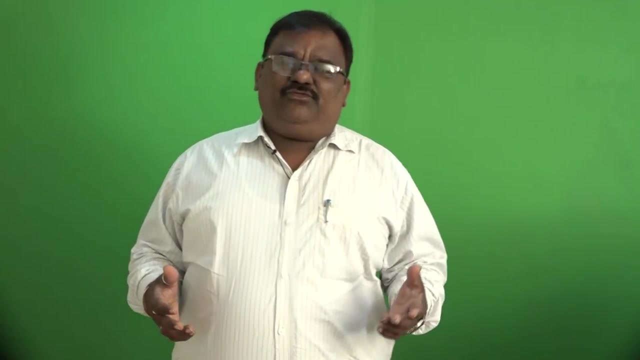 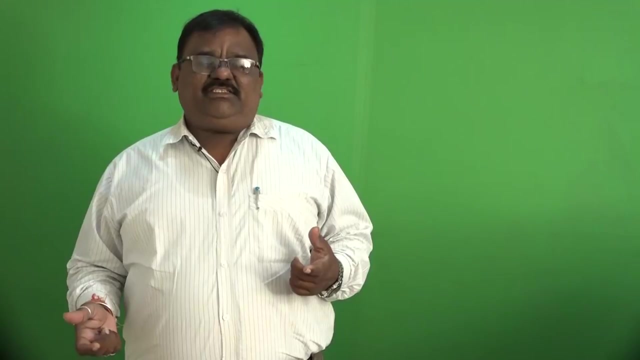 genes we learned about the molecules in also we can in environmental chemistry in our content. the main content is also ethics, ethics, policy of rules, regulation of the environment. without know the policy ethics, how we can save our environment and the world in our environment chemistry we can also. we can also just develop ecotourism, ecotourism. what is ecotourism? to just generate. 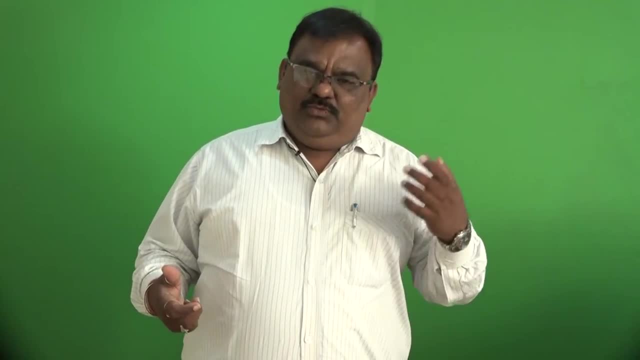 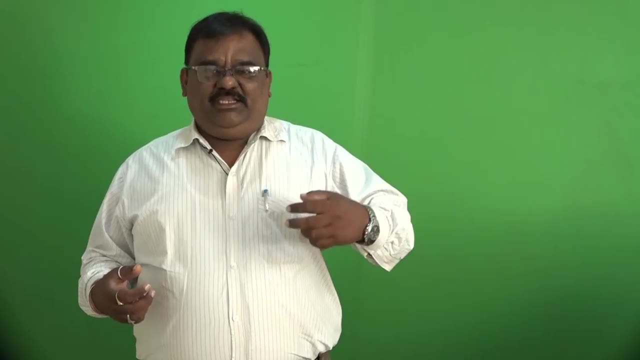 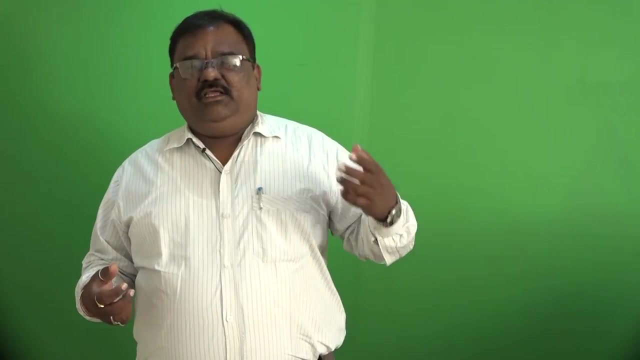 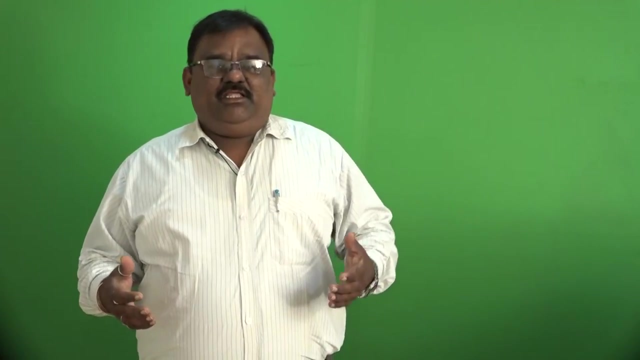 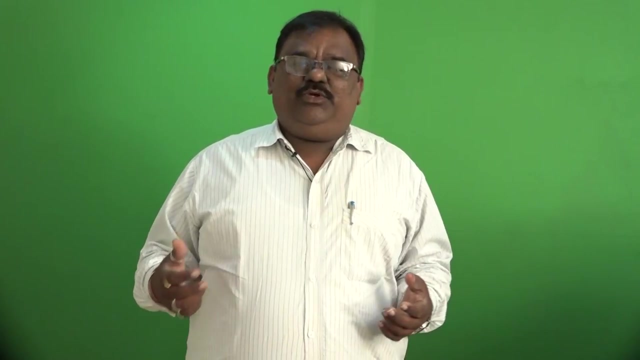 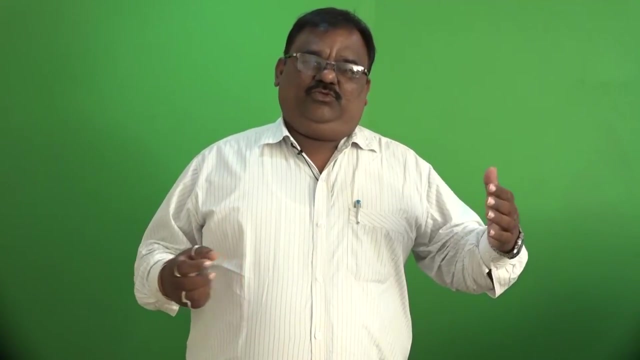 conserve this type of natural places to how develop this we can easily just included in our content in in green chemistry we also develop the several drugs, several manufacturing molecules, how we can do this. so in our environmental chemistry the main aim to develop the student close relation environment, how student deal with the problem of this type of globally so we can solve this to. 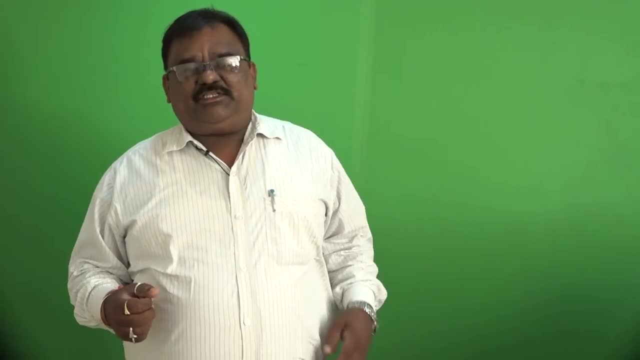 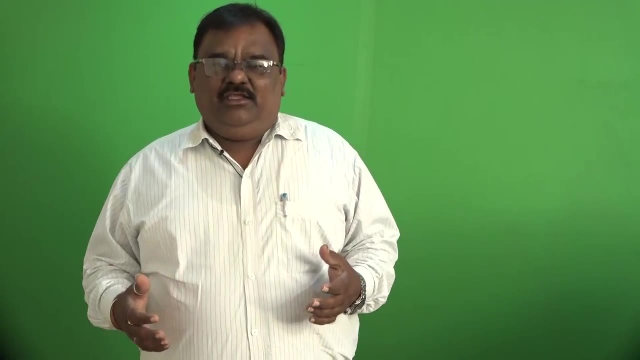 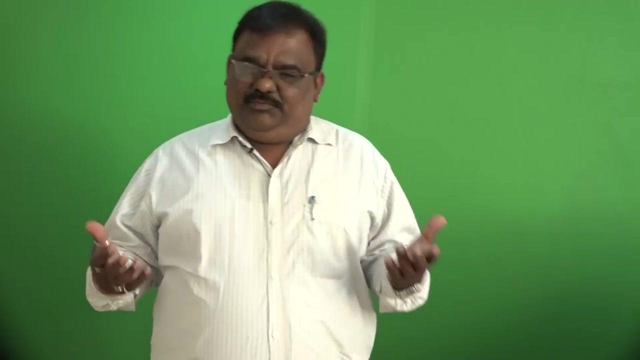 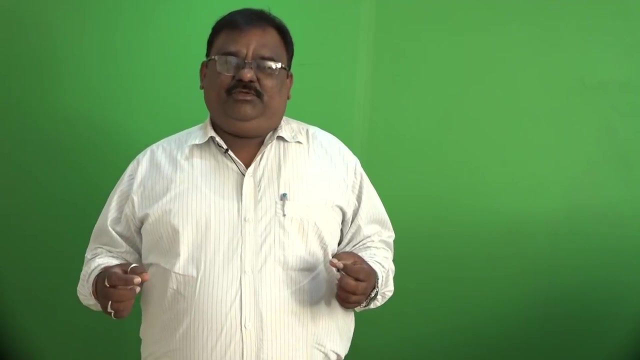 include our inner content. so in environmental chemistry, just student developed to a professionally, professionally carrier, we developed the student, our we want to our student develop the research facility, research, research tendency, how this is. so the content is the purely developed c to this type of matter. so in environmental chemistry we 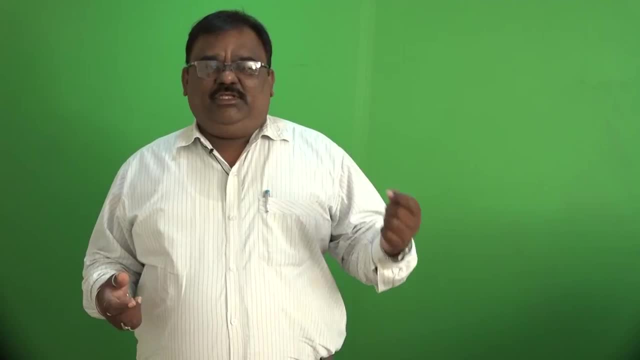 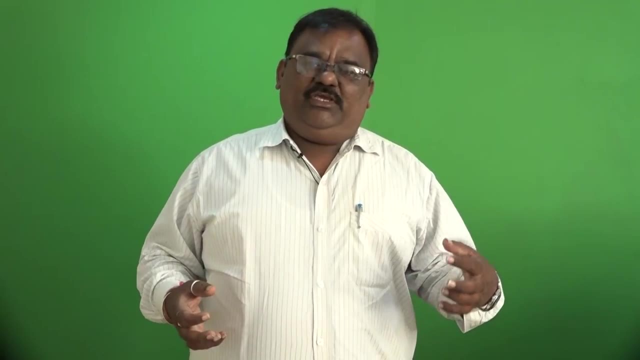 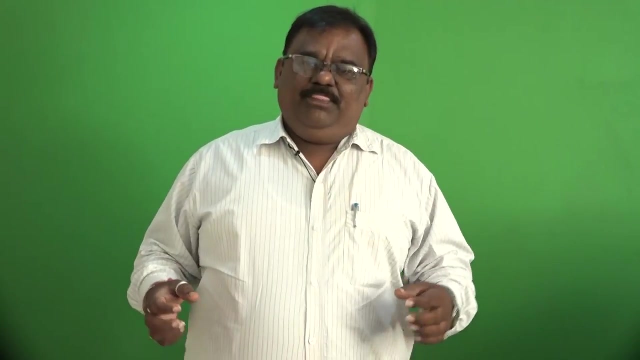 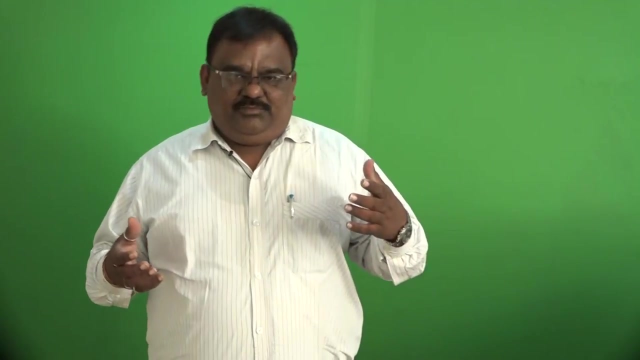 just provide to student from water pollution, from general definition to the act and policy of the environment. so in this course we conclude all this type of basic and the fundamental problems in this type of courses. so this course definitely provide a student a bit better platform, a better places and definitely student just go to the better places to just 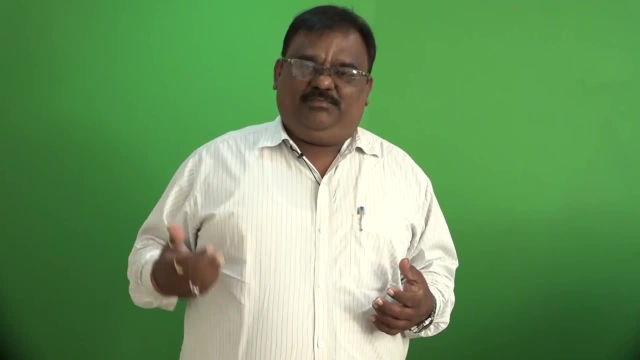 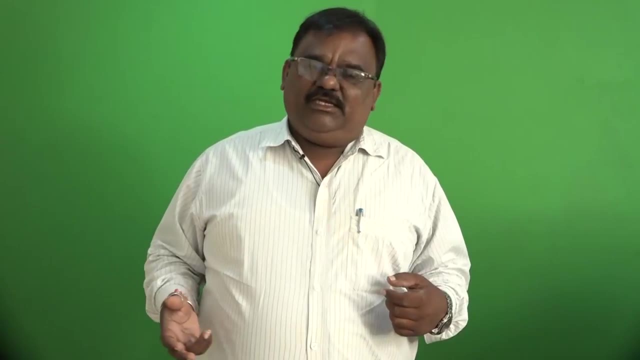 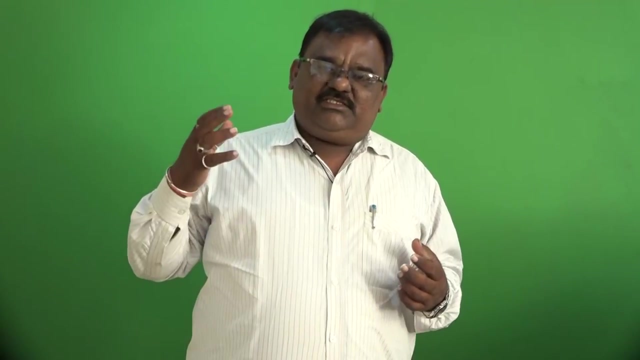 absorb the that place. so our environmental chemistry syllabus is: not only we want to just give the degree to the student, we want to just learn. we want to just give the all types of modern just facility, all modern techniques like a double as, like lms and other things like that and so on.